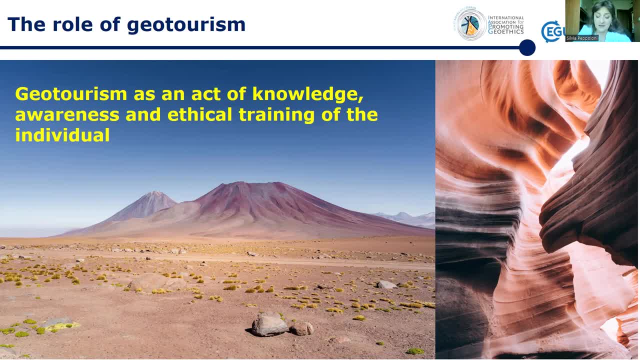 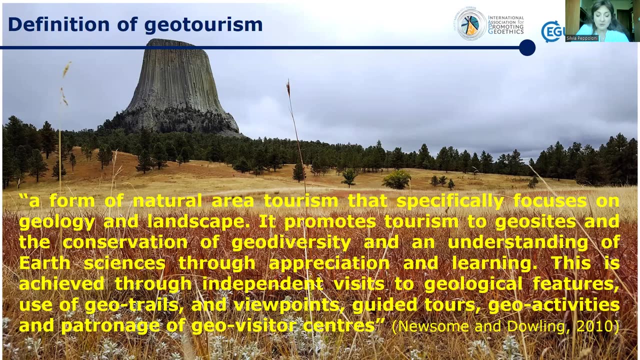 function for those who experience it, redeveloping geotourism as an act of knowledge, awareness and ethical training for the individual. Among the various definitions of geotourism, we refer to that one. This definition clarifies what geotourism consists of, what are its purposes, the activities. 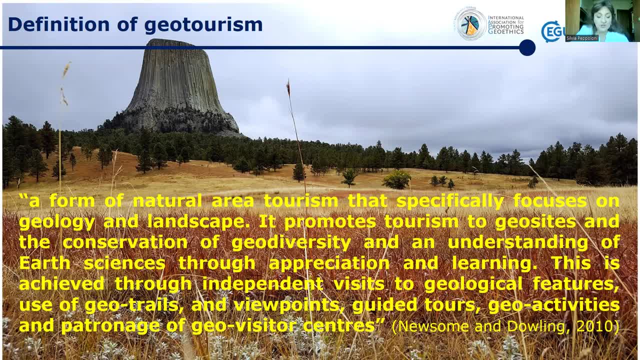 that allow its use and the different forms in which it can be expressed. The reference to the concept of conservation of geodiversity is significant because it gives to geotourism a meaning that goes beyond the scientific, aesthetic, cultural and regenerative use. 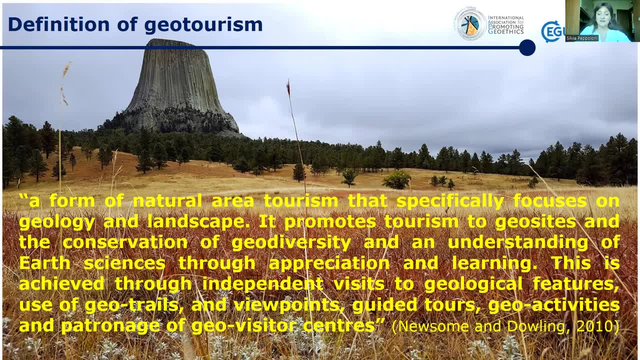 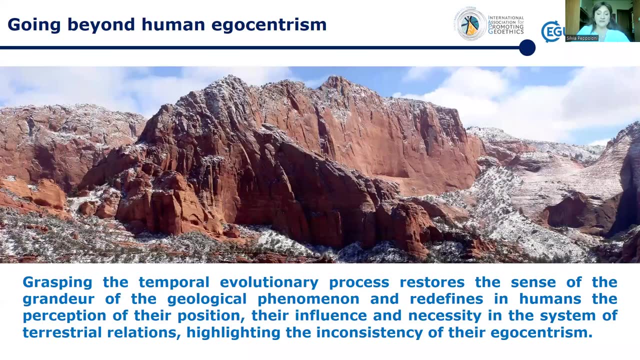 of the landscape by the individual. In fact, it necessarily becomes a proposal of concrete action in defense of those abiotic components that constitute its main objects of interest. A first consideration: The geotouristic experience is rich and satisfying not only when it captures. 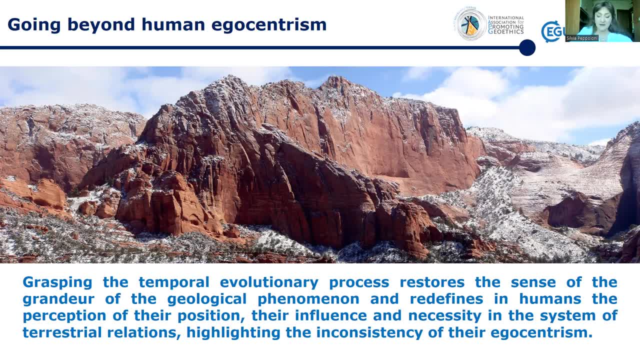 the final result when it grasps the final forms produced by geological events, such as an outcrop, geological landscape, a fossil or a mineral, but also when it understands the entire historical process that created that form: The geodynamic, lithogenetic or morphological process that 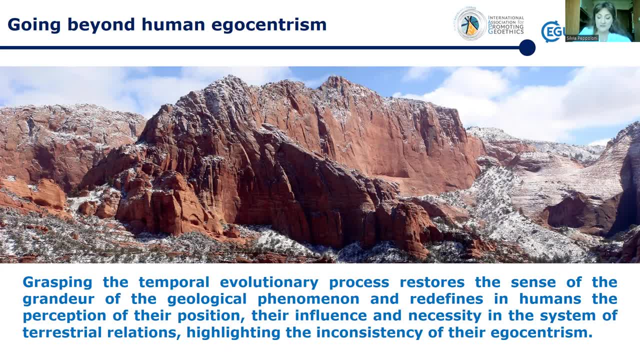 ultimately intersects and merges with the history of the geological process. The geological process is the basis of humanity itself. Grasping the temporal evolutionary process restores the sense of the grandeur of the geological phenomenon and redefines in humans the perception of their position on the earth, their influence and necessity in the system of terrestrial. 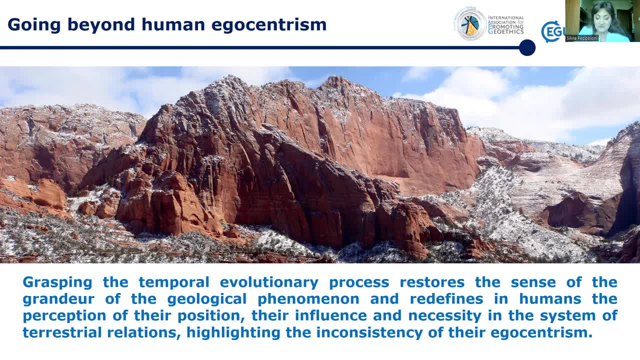 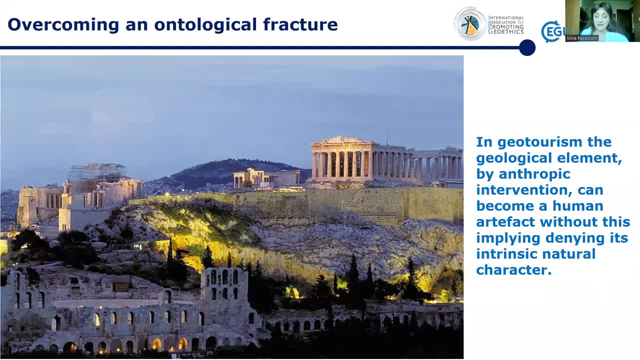 relations, highlighting the inconsistency of their egocentrism. A second consideration: Geotourism can take place in the context of the geological process. The geological process is not only in natural areas, but also in human-modified environments. This does not. 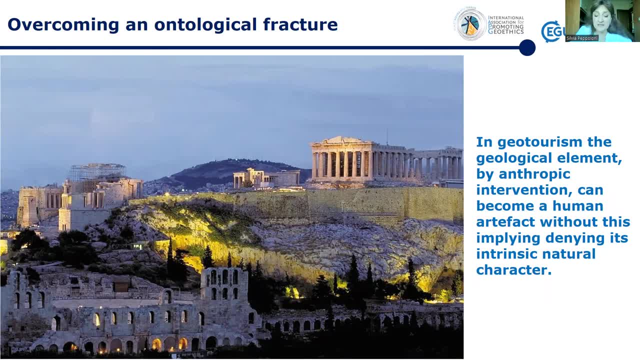 take away value and significance from strictly naturalistic tourism, but rather extends it to those geological elements that, due to human intervention, have been incorporated into the cultural, artistic, architectural and urbanistic heritage, thus creating an ideal geotourism. 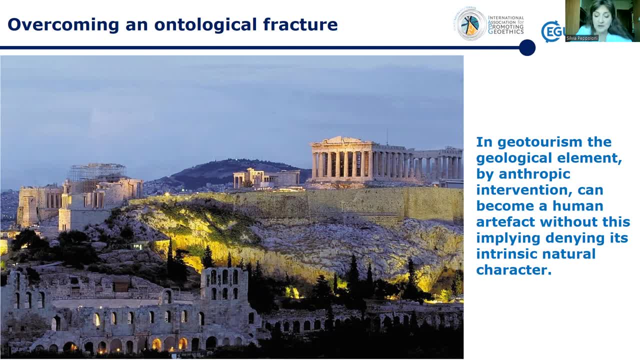 The geological process is a bridge to overcome the ancient ontological fracture between human beings and the natural environment, between culture and nature. In other words, in geotourism, the geological element by anthropic intervention becomes a human artefact, without these implying. 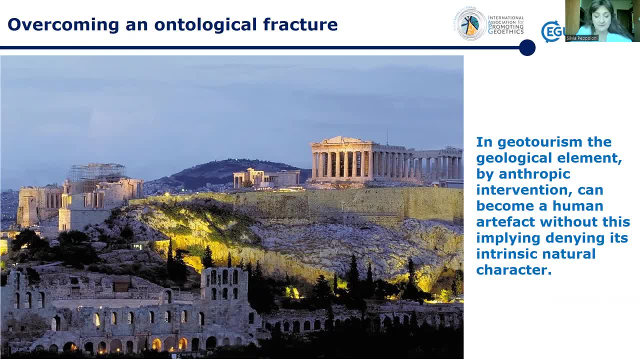 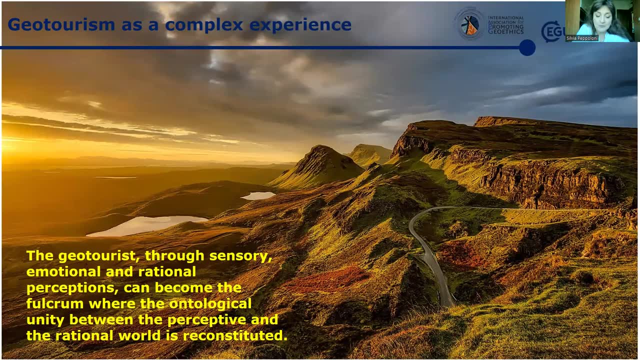 denying its intrinsic natural character. Therefore, geotourism is much more than just looking at landscapes. Geotourism allows you to go beyond aesthetic appreciation, beyond the recreational, intuitive, relaxing moment, to become an authentic, formative, educational tool for the human being. 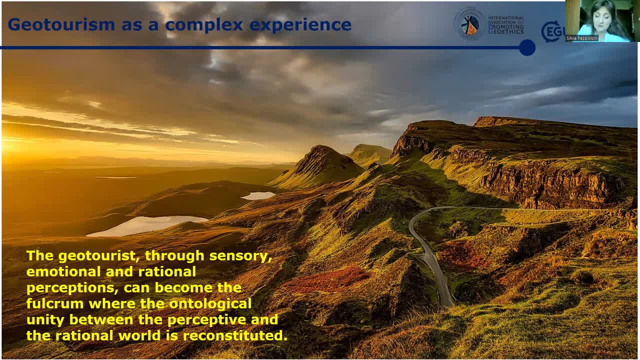 Moreover, while geotourism provides knowledge of the great geological processes such as crustal movements, aesthetic changes, paleogeographic evolution through the observation of fossils and rocks, at the same time it favors in the geotourist a reflection on their own nature, the awareness of their own finitude as human beings. 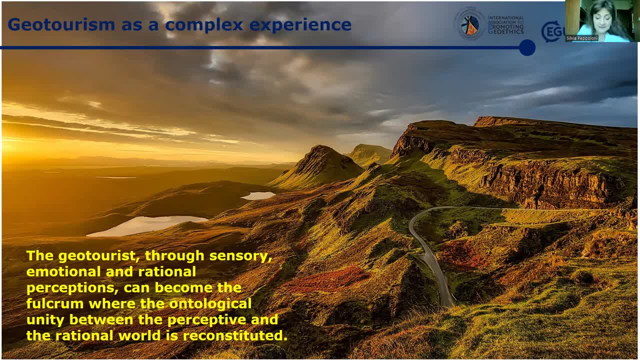 and on the transience and vulnerability of nature. Geotourism has the potential to perceptively grasp the unity of the elements and rationally place them within a systemic interpretative framework. Here the geotouristic experience becomes a moment of unity between sensory perception and rational mediation. 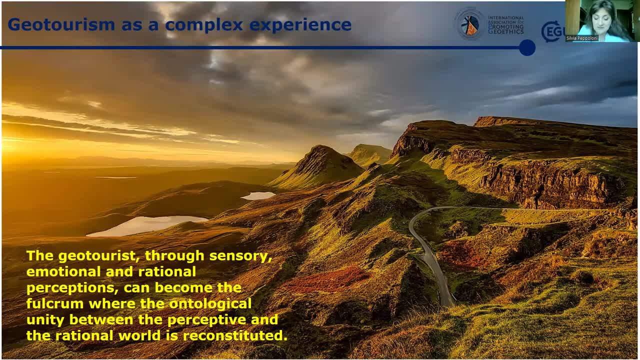 which can allow us overcoming the reductionist perspective of modern science. Through sensory, emotional and rational perceptions, the geotourist can become the fulcrum where the ontological unity between the perceptive and the rational world is reconstituted.